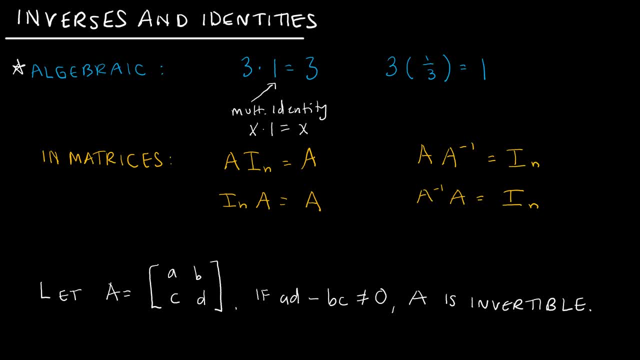 value x takes on. if I multiply anything by 1, I end up back at that value. The reason I bring that up is because I know that the inverse of a matrix is an integral of my original value. ____________________________ Security: if a single figure f is made black, if a single figure c is made white and 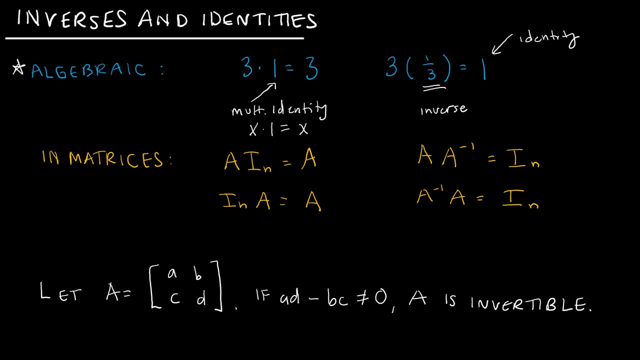 represented in black, then if we do theillos out by vibrations, then if we multiply by the samaa, we get the entire idea. So this is my version of a structure. simply referring today are three podrichromess: ______________. denote that x to the negative 1, that tells us that that's the inverse is equal to the identity. 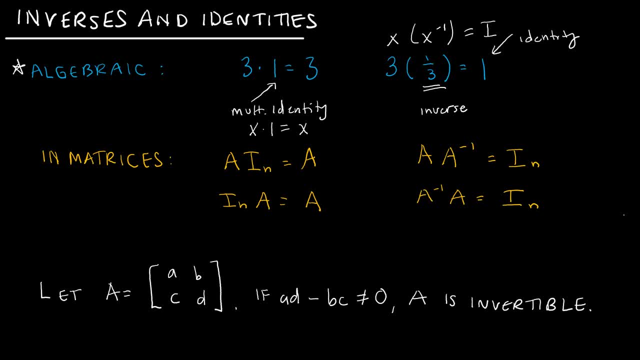 So now let's take a look at matrices instead of an algebraic problem In matrices. I have matrix A, and matrix A multiplied by the inverse matrix should get me back to A. And notice, with the inverse I can actually multiply those two in either order and end up back at A. So just 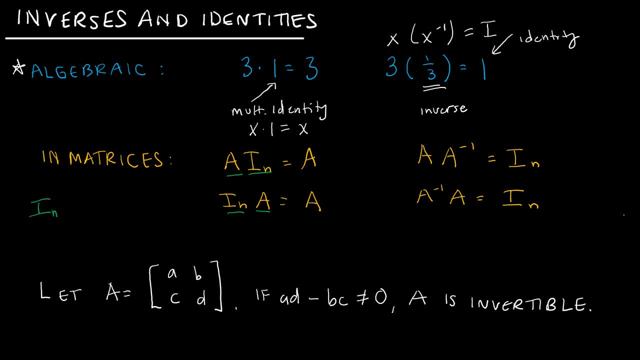 as a refresher in case you have forgotten, the inverse matrix is a square matrix. it's a square diagonal matrix with 1 in the diagonal. So 1, 0, 0, 0, 1, 0, 0, 0, 1 would be the identity matrix. 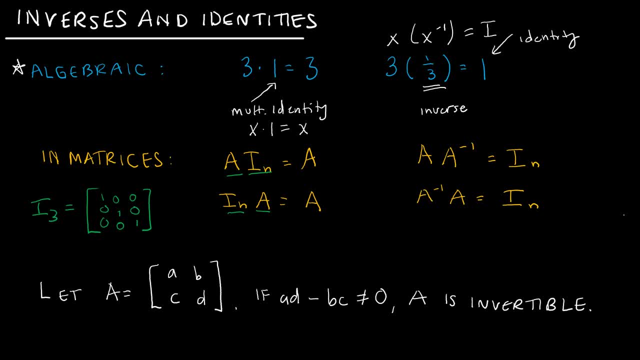 for 3, because there's 3 rows, 3 columns. So, looking at kind of similarly to the way that we looked at it in algebraic terms, if I took A multiplied by the inverse of A and notice that same notation, or if I took the inverse of A times A, 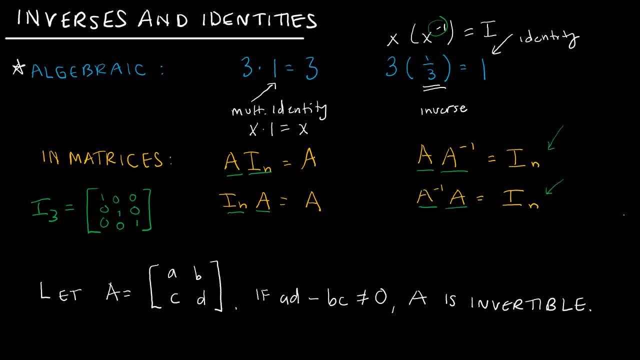 either way, I should end up back at the identity matrix. A bunch of 1s in a diagonal with the rest 0s. So that's what an inverse is and obviously what an identity is. Notice at the very bottom. I have sort of a definition here and it's only part of a definition. we'll finish. 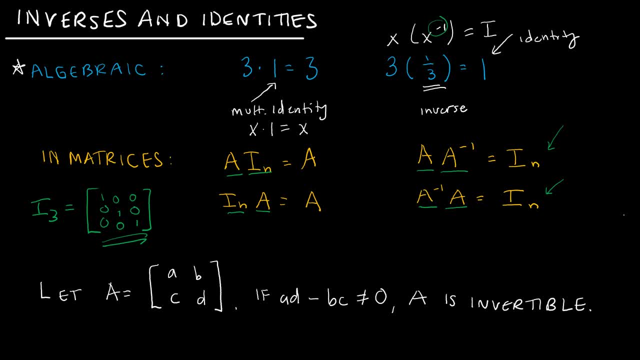 the rest on the next page. But I wanted to talk about how do I know a matrix is invertible. Well, this is obviously specific to a 2 by 2 matrix. To know if a 2 by 2 matrix is invertible. 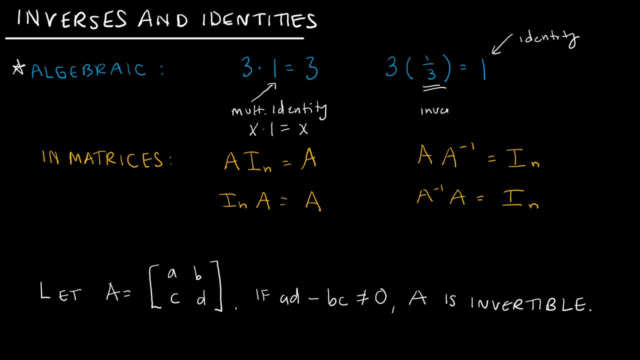 something called an inverse, And an inverse is a value that you would multiply by your original value to get back to the identity. So, symbolically, I would say that x multiplied by the inverse- and this is how we denote to note that x to the negative 1, that tells us that that's the inverse- is equal to the identity. 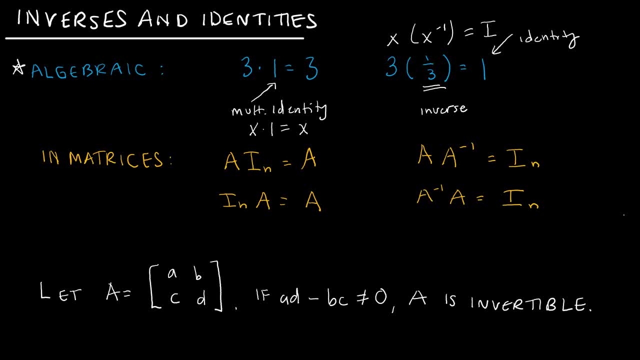 So now let's take a look at matrices instead of an algebraic problem In matrices. I have matrix A, and matrix A multiplied by the inverse matrix should get me back to A. And notice, with the inverse I can actually multiply those two in either order and end up back at A. So just as a. 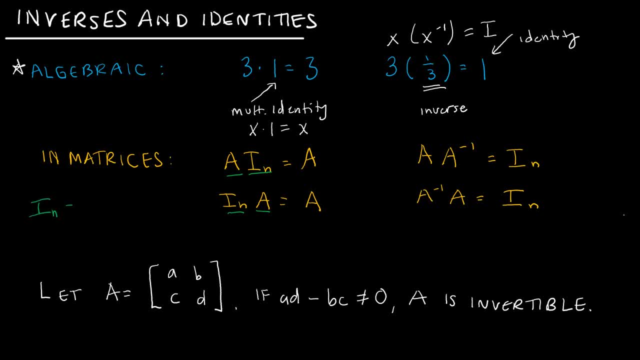 refresher in case you have forgotten. the inverse matrix is a square matrix. It's a square diagonal matrix with one in the diagonal, So one in the diagonal, one in the diagonal and one in the diagonal. So one in the diagonal and one in the diagonal. So one in the diagonal and one in the 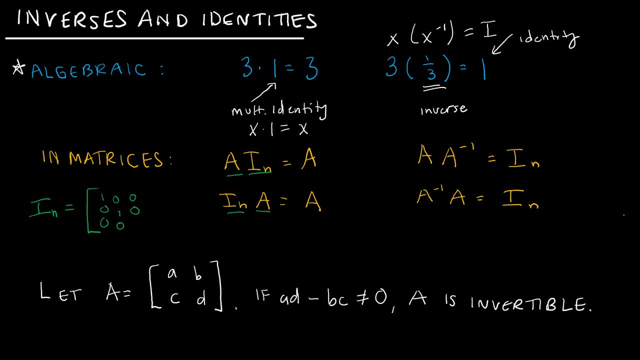 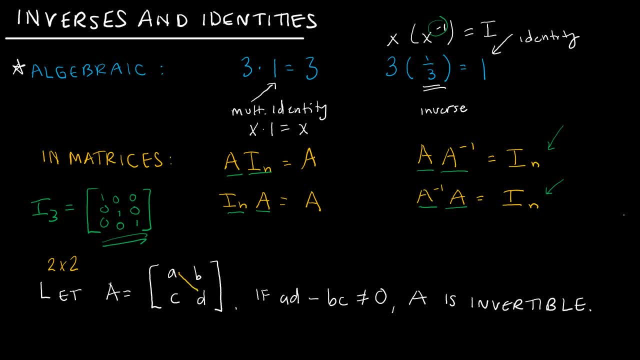 I would take A times D, which is that first diagonal, minus B times C, which is the second diagonal. and if that is not equal to 0, then A is invertible. This value is called the determinant of A, and that's how we denote that. So the determinant of A is AD minus BC. So we'll talk. 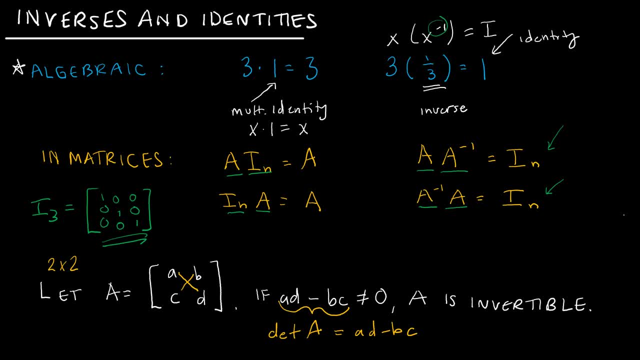 a little bit more about that on the next slide. but again, this is: how do you know? it's invertible. You would find that in the first diagonal and then you would find that in the second diagonal. and the determinant: make sure the determinant is non-zero. 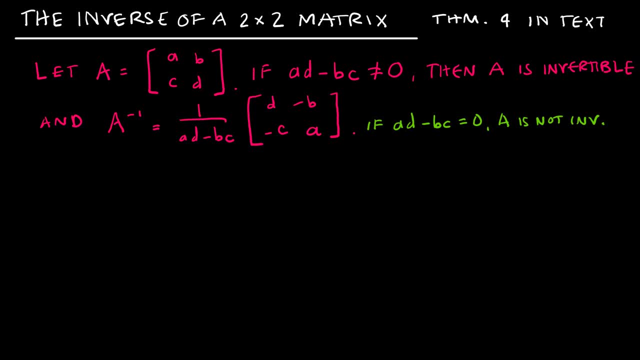 Looking specifically at a 2 by 2 matrix. I've now given you the rest of this definition or theorem. The theorem says that the inverse of a 2 by 2 matrix can be found first by verifying that AD minus BC is not equal to 0, and again, that is the part that we talked about already. 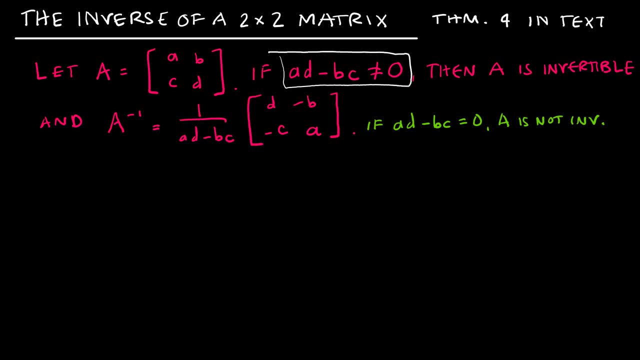 We need that determinant to not be equal to 0, therefore, A is invertible. and then it tells us that A inverse can be found using this formula. So notice: this formula is really 1 over the determinant of A, because we talked about that being the determinant. 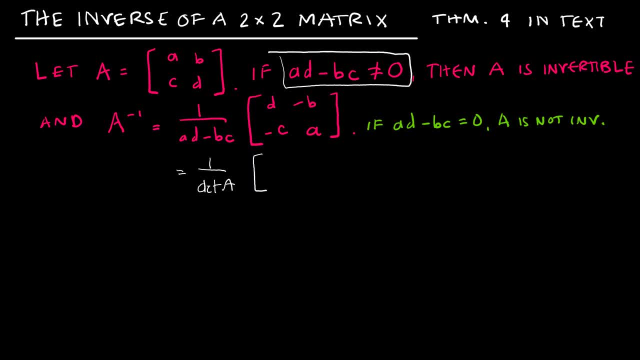 and then notice what happened to the values A and D. just switched places so it started as A here and D here. To find the determinant, I'm going to switch the first diagonal and notice the second diagonal. B and C are in the correct spot, but they're negatives. 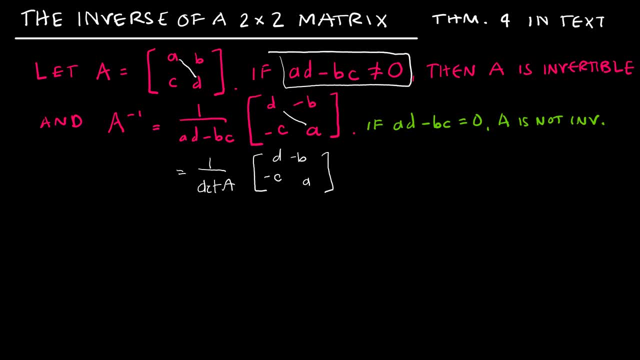 So the first diagonal, I'm going to change the values with each other, and the second diagonal, I'm going to change the signs. Now, before we actually use this formula to find the inverse of a 2 by 2 matrix, let's just talk about the fact that it is going to work. So I know. 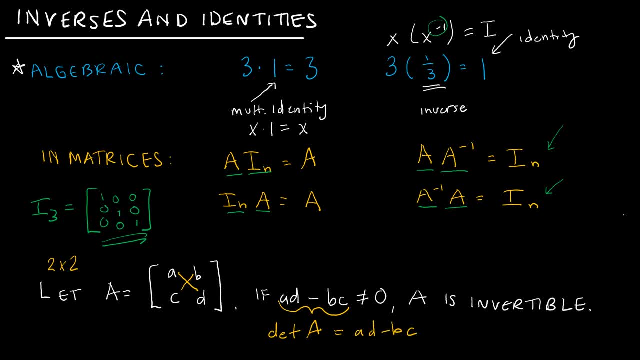 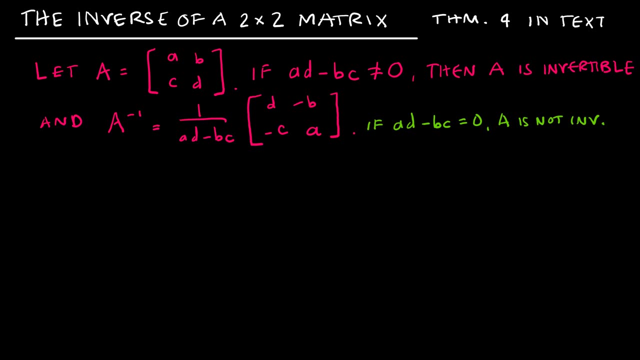 diagonal. So one in the diagonal and one in the diagonal. So one in the diagonal and one in the. again, that is the part that we talked about already. We need that determinant to not be equal to zero. Therefore A is invertible, And then it tells us that A inverse can be found. 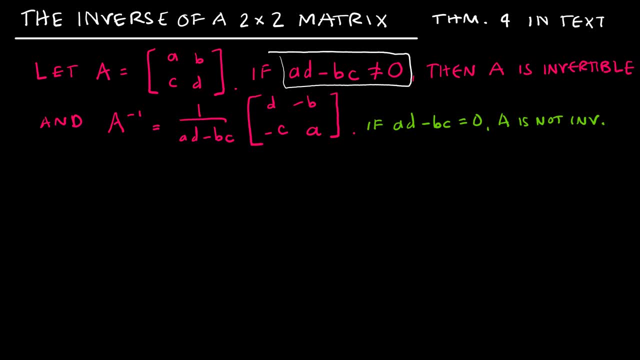 using this formula. So notice this formula is really one over the determinant of A, because we talked about that being the determinant. And then notice what happened to the values A and D. just switched places. So it started as A here and D here. 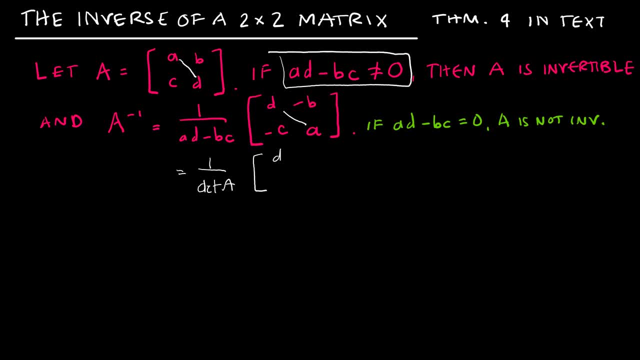 To find the determinant, I'm going to switch the first diagonal And notice the second diagonal: B and C are in the correct spot, but they're negatives. So the first diagonal, I'm going to change the values with each other, And the second diagonal, I'm going to change the signs. 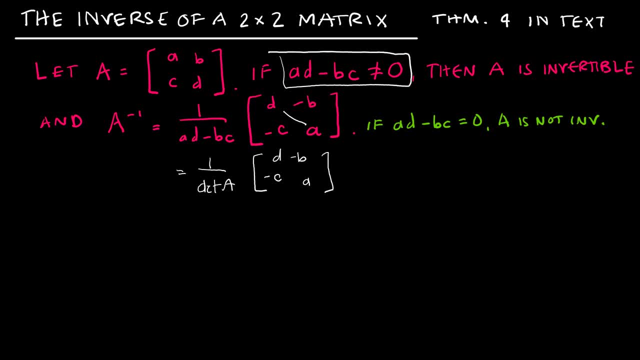 Now, before we actually use this formula to find the inverse of a two by two matrix, let's just talk about the fact that it is going to work. So I know, based on what we talked about before, that A times A inverse should give me. 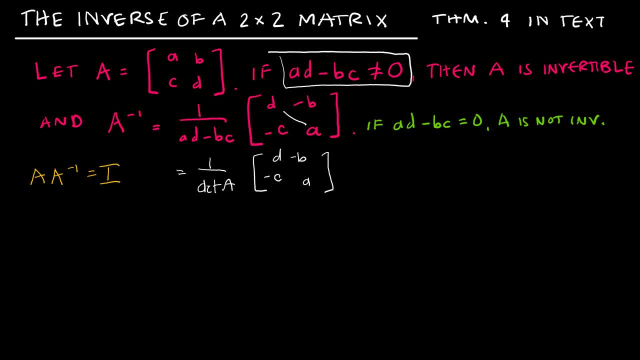 the identity. So let's do that symbolically: A, B, C, D times. A inverse should give me the identity. So let's do that symbolically: A, B, C, D times, A inverse should give me the identity. So let's do that symbolically: A, B, C, D times. 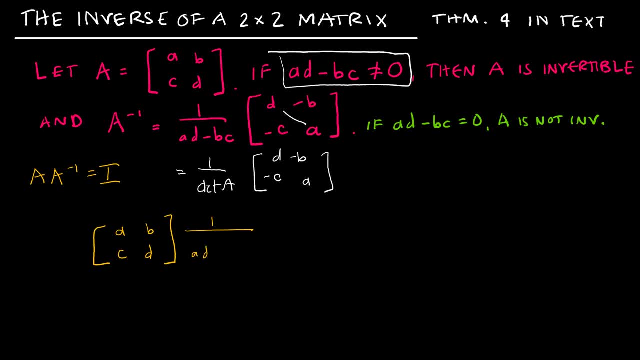 one over A, D minus B C multiplied by D minus B minus C A, So that's A times A inverse. And supposedly, if I do all of this work, I shouldn't end up at the identity And remember that the identity in this case would be one zero zero one. So let's do that symbolically. 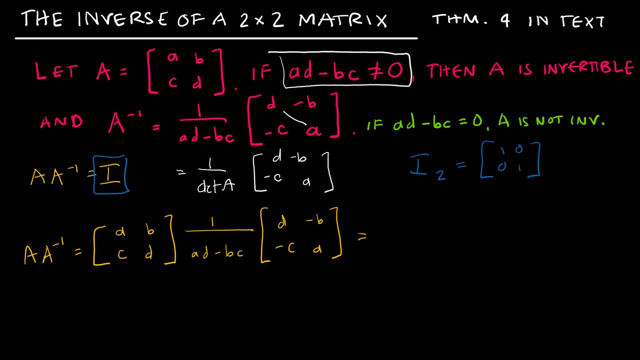 Let's just test our mathematical ability and see if that's what we get. If I take- and I'm going to just make the computations easier by popping this to the other side, So we know that's a scalar, and a scalar can be put on one side or the other. 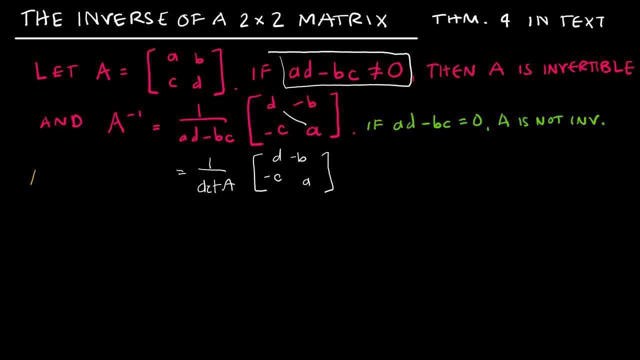 based on what we talked about before, that A times A inverse should give me the identity. So let's do that symbolically: A B, C D times 1 over AD minus BC, multiplied by D minus B minus CA, That's A times A inverse And supposedly, if I do all of this work I shouldn't end up at 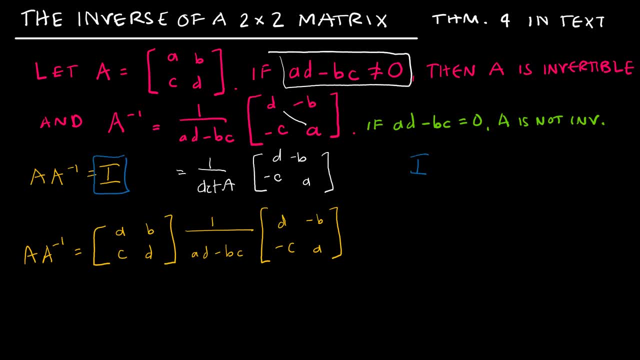 the identity, and remember that the identity in this case would be 1, 0, 0, 1.. So let's just test our mathematical ability and see if that's what we get. If I take- and I'm going to just make- 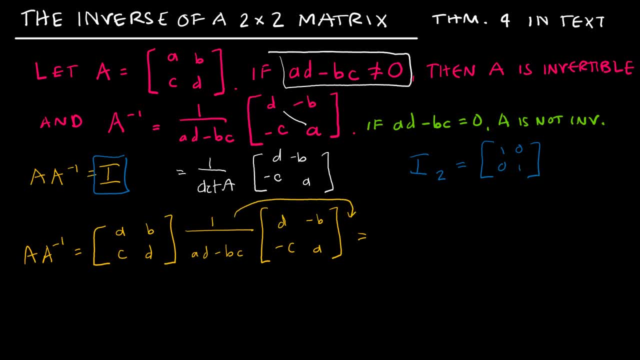 popping this to the other side. So we know that's a scalar, and a scalar can be put on one side or the other and it's not going to change it. We talked about that in our last video, So I'm going to focus first on just multiplying the two matrices together and then, at the end, I'll 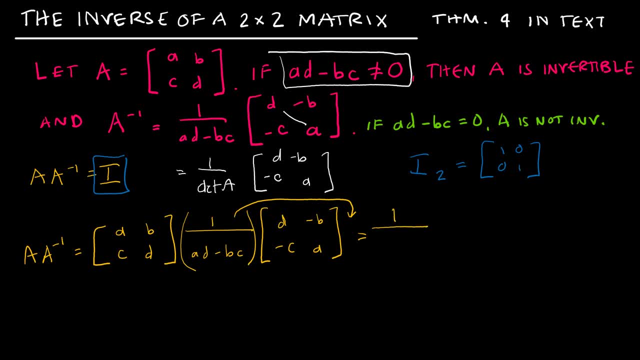 multiply by that scalar. So I'm going to put the scalar out front and I'm going to multiply the matrices. So I'm going to take my first row: A, B times my first column. So that's A times D plus B times negative C. So I'm just going to 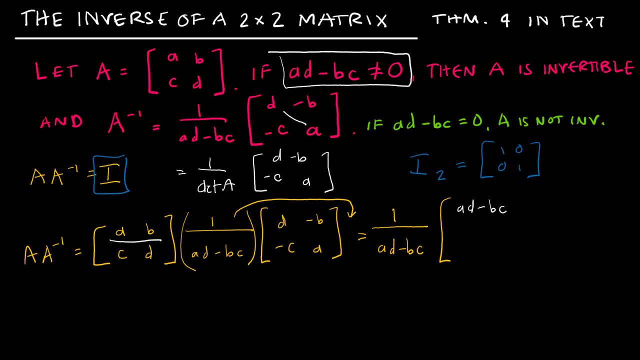 change that to minus BC And then first row times second column would be negative A B plus B A. Let me go ahead and switch back to yellow for that other row Bracket, And then I'm going to take my second row and do the same thing. So C times D plus D times. 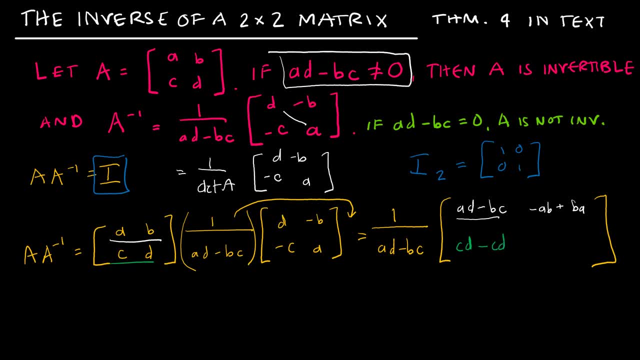 negative C, So again minus CD, And then C times negative B, plus D times A. So let's do a little bit of cleanup here. So I still have this scalar which AD minus BC, And I could put that at the beginning or the end. 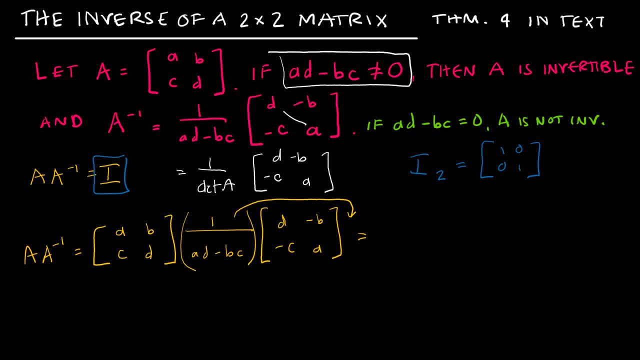 and it's not going to change it. We talked about that in our last video. So I'm going to focus first on just multiplying the two matrices together And then, at the end, I'll multiply by that scalar. So I'm going to put the scalar out front. 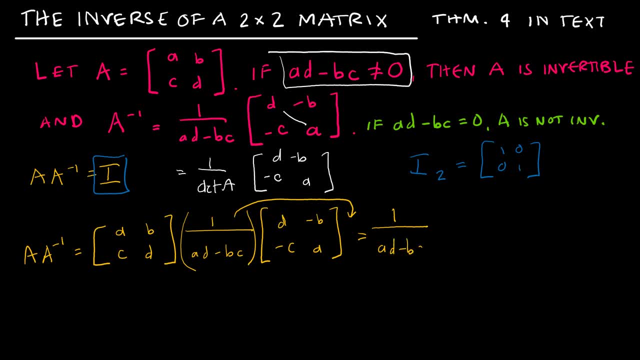 And I'm going to multiply the matrices. So I'm going to take my first row, A, B times my first column, So that's A times D plus B times negative C. So I'm just going to change that to minus B C And then first row times, second column would be negative C. 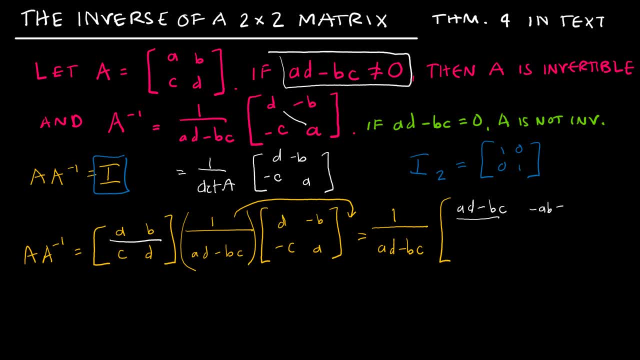 So I'm going to take my first row, A, B times my first column. So that's A times D plus B times, negative ab plus ba. Let me go ahead and switch back to yellow for that other bracket, And then I'm going to take my second row and do the same thing, So c times d plus d times. 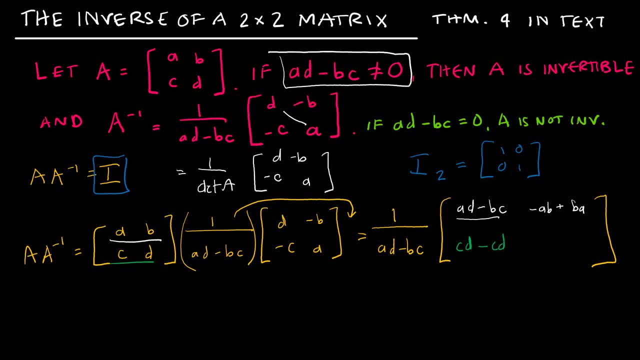 negative c, so again minus cd, and then c times negative b plus d times a. So let's do a little bit of cleanup here. So I still have this scalar which ad minus bc, and I could put that at the beginning or the end, because it's a scalar and it doesn't matter. 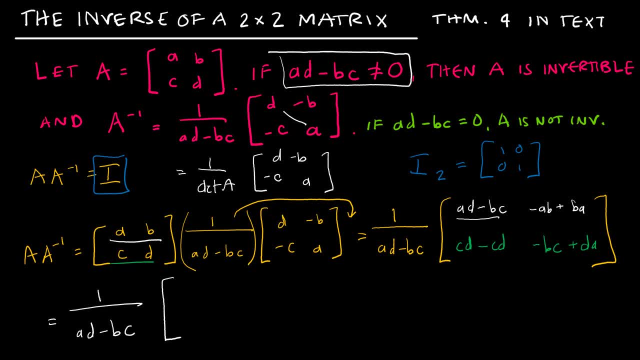 But let's do a little bit of cleanup. ad minus bc is just ad minus bc. That my second term. minus ab plus ba. well, these are the same thing, ab and ab. So I have minus ab and positive ab, which gives me zero, And 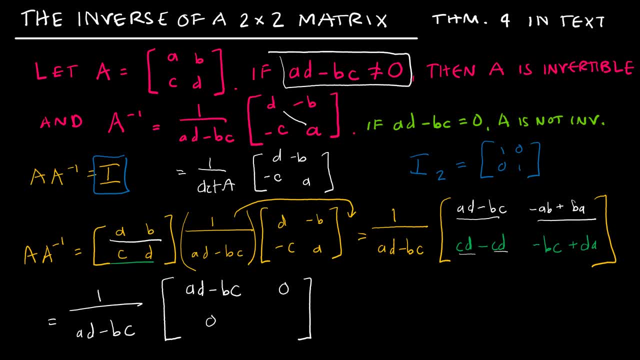 then cd and cd. that's zero. And then I'm just going to change the order here. I'm going to put ad first, so ad minus bc. Okay, Okay, Okay. And we can see now, if I take each term multiplied by my scalar, that I'm going to end up with. 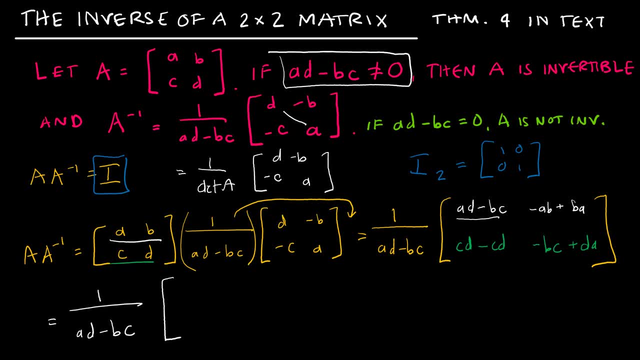 because it's a scalar and it doesn't matter. But let's do a little bit of cleanup. AD minus BC is just AD minus BC. That my second term. minus AB plus BA. well, these are the same thing, AB and AB. So I have minus AB and positive AB, which gives me zero, And then CD and CD. that's zero. So I have minus AB and positive AB, which gives me zero, And then CD and CD, that's zero. So I have minus AB and positive AB, which gives me zero, And then CD and CD, that's zero. 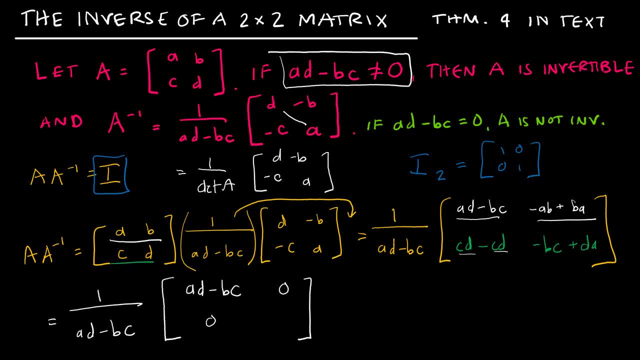 And then CD and CD- that's zero. And then CD and CD- that's zero. And then I'm just going to change the order here. I'm going to put AD first, So AD minus BC, And we can see now if I take each term. 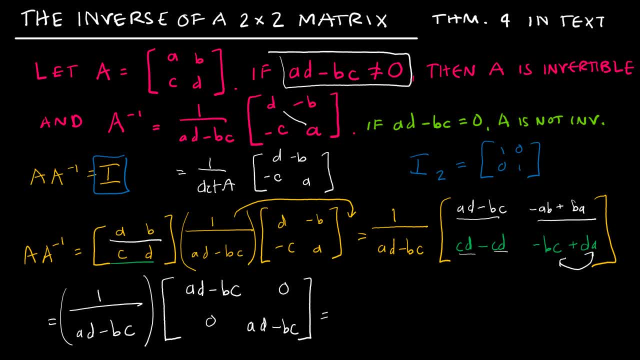 multiplied by my scalar, that I'm going to end up with AD minus BC over AD minus BC, And that's just zero, and that's just zero, and that's AD minus BC over AD minus BC, And that gives me 1, 0, 0, 1.. And therefore we have shown this is not a proof. 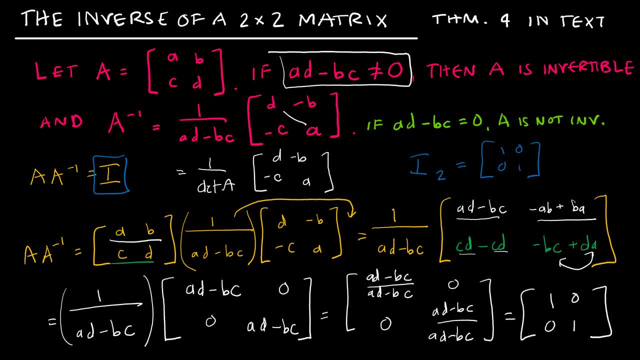 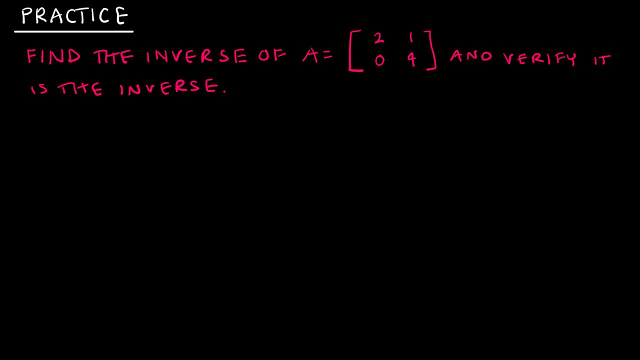 but we have shown that will in fact give us the identity. Here's a practice for us to do together. It says: find the inverse of A and verify: it is the inverse. So again, I probably should have rewritten that formula for you, since I doubt that you have it. 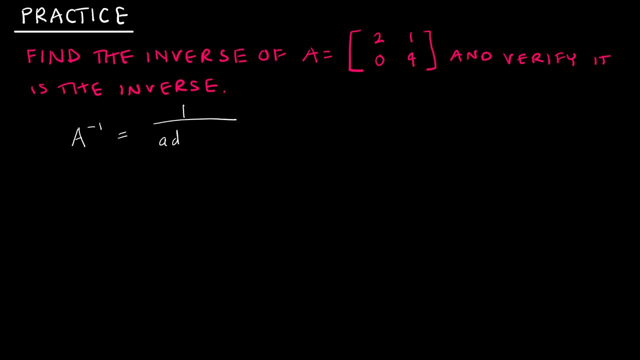 memorized by now. So we have AD minus BC And remember D and A switched places and B and C switched signs. So that means again my original matrix A is ABCD. So I'm just going to use this formula, I'm going to take 1 minus and then AD would be 2 times 4.. 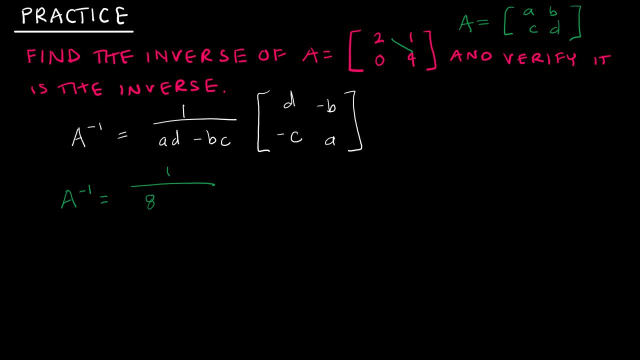 Now I'll just go ahead and write 2 times 4.. So we remember where everything came from: 2 times 4 minus 0 times 1.. And then remember how I find this. I'm going to take these two and switch places. 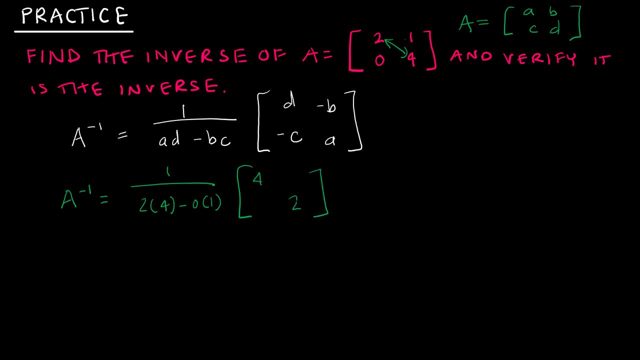 So the 2 and the 4 will switch places, and the 1 and the 0 will switch signs. So negative 1, and obviously there's no such thing as negative 0, so it's just 0.. Now I'm just going to do the. 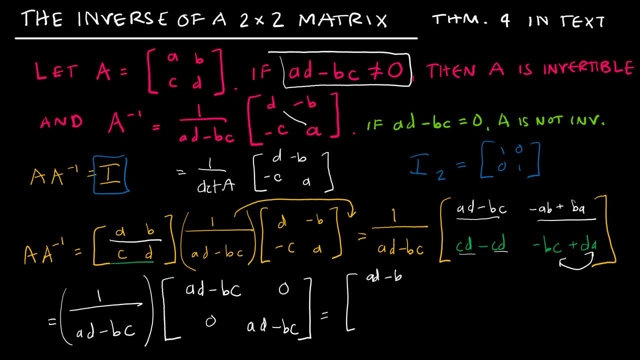 ad minus bc over ad minus bc, And that's just zero, and that's just zero, and that's ad minus bc over ad minus bc, And that gives me one zero, zero one. And therefore we have shown- this is not a proof, but we have shown- that will in fact give us the identity. 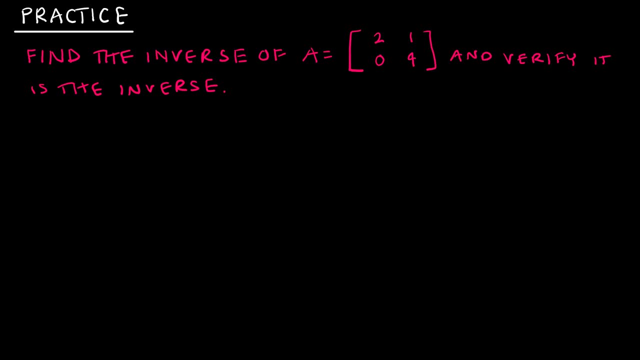 No, Here's a practice for us to do together. It says: find the inverse of A and verify: it is the inverse. So again, I probably should have rewritten that formula for you, since I doubt that you have it memorized by now. So we have ad minus bc, and remember d and. 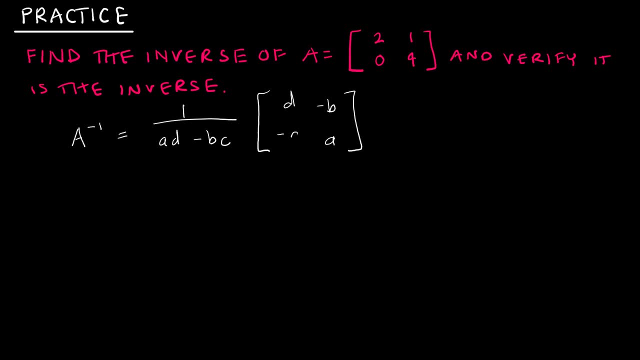 a switched places and b and c switched places. No switched signs. So that means again my original matrix A is ABCD. So I'm just going to use this formula. I'm going to take 1 minus and then AD would be 2 times 4.. Now let's go ahead and write. 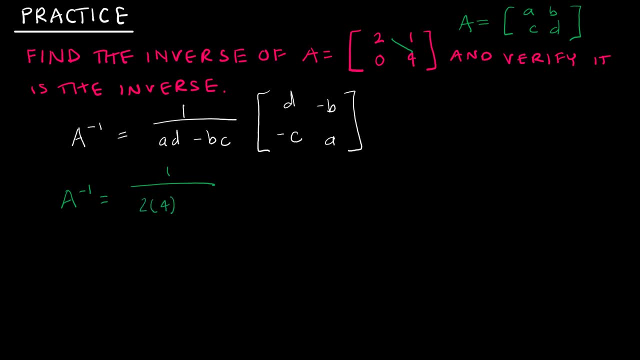 2 times 4.. So we remember where everything came from: 2 times 4 minus 0 times 1.. And then remember how I find this. I'm going to take these two and switch places. So the 2 and the 4 will switch places and the 1 and the 0 will switch signs. So negative 1,. 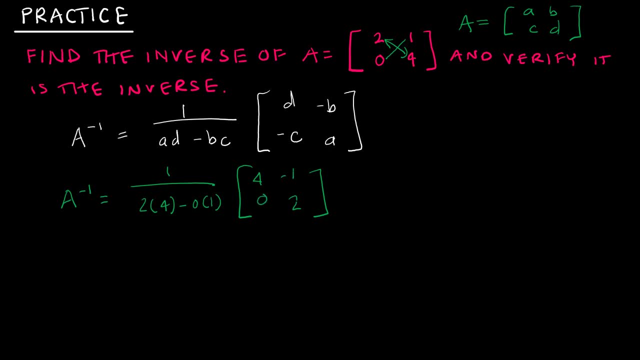 and obviously there's no such thing as negative 0, so it's just 0.. Now I'm just going to do the computation. So 1 over that's 8 minus 0, so 1 eighth times. oops, I'm going to take. 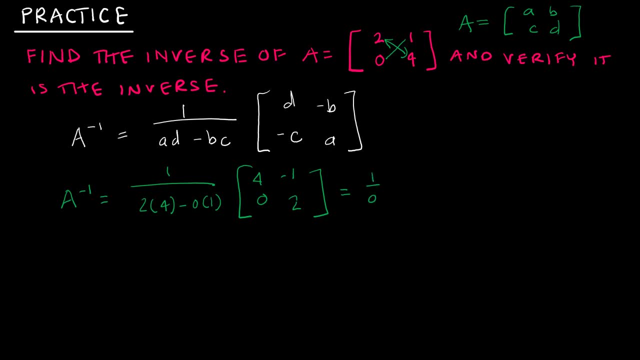 up a lot of room there. so let's try this again: 1, eighth and then 4, negative 1, 0, 2.. So if I take an eighth of each of those- and I'm going to go ahead and take an eighth and reduce, so 4 over. 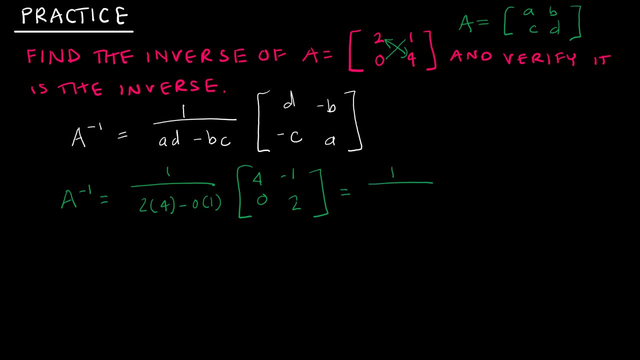 computation. So 1 over, that's 8 minus 0,. so 1 eighth times. oops, I'm taking up a lot of room there, so let's try this again: 1 eighth and then 4 negative, 1,, 0,, 2.. So if I take an eighth of each, 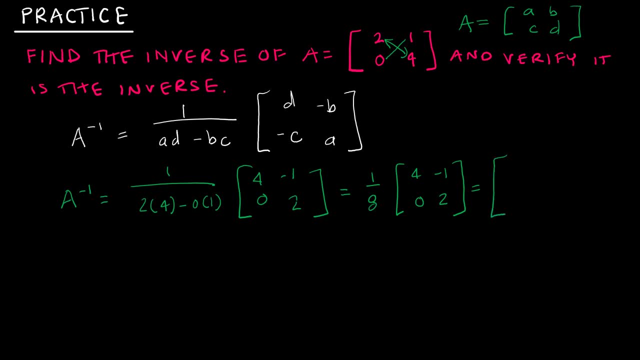 of those, and I'm going to go ahead and take an eighth and reduce. So 4 over 8,, which reduces to 1 half negative, 1 over 8.. 0 over 8, which is 0, and then 2 over 8,, which is 1 fourth. So that is my inverse matrix for A. 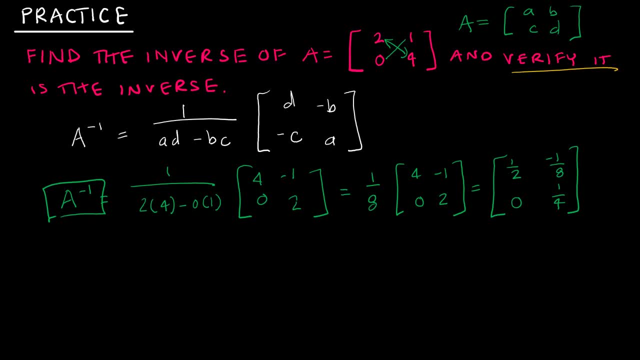 Now I'm going to verify. it is the inverse. So to verify, I'm going to take A times A inverse and that means I have 2, 1, 0, 4.. So I'm going to take A times 1 half negative, 1 eighth, 0, 1 fourth, and again you can feel free. 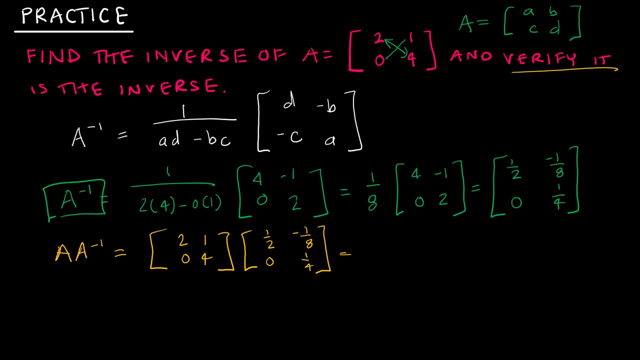 to help yourself with a calculator, but it's good for you to do mental math, So if you can do it without a calculator, that's what you should do. So here we go. I'm going to take 2 times 1 half. 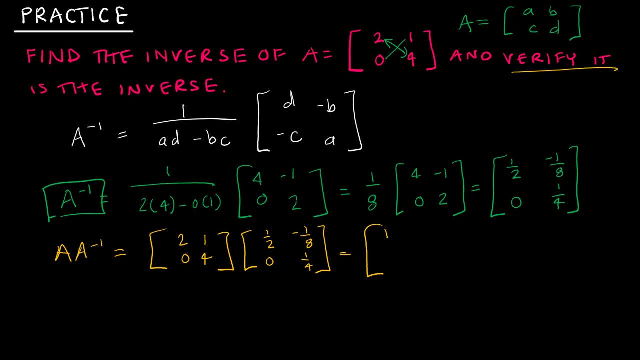 which is 1, and 1 times 1 fourth. Hold on, Nope, just kidding. 1 times 0,, which is 0. I knew that was wrong. And then I'm going to take 2 times negative 1 eighth, which is negative 1 fourth. 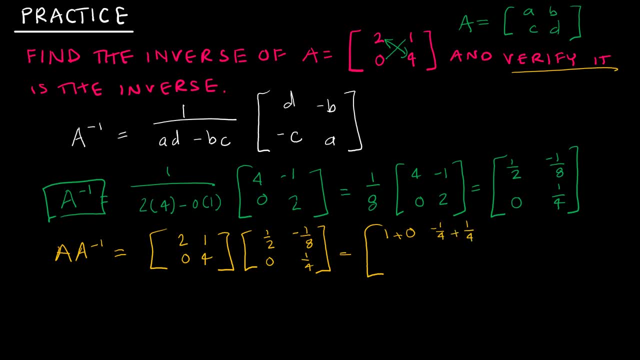 and I'm going to take 1 times 1- fourth, which is 1, fourth, And that was my first row times each column, and now I'm going to take my second row, So 0 plus 4 times 0,, which is 0, and then 0 times 1- eighth, is 0,. 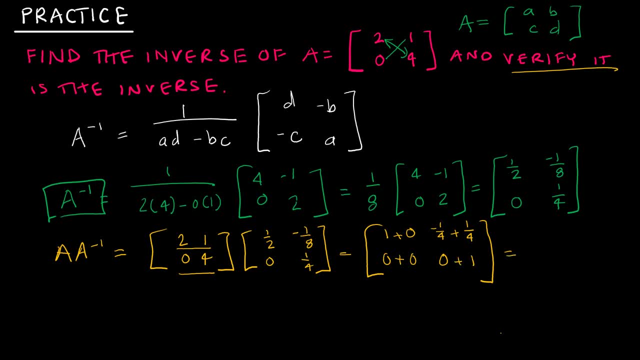 I'm sorry. 4 times 1, fourth is 1.. So what did I end up with? 1, 0, 0, 1, which is the identity matrix. Now, just for fun, because math is so much fun, let's take A inverse times A and verify that we. 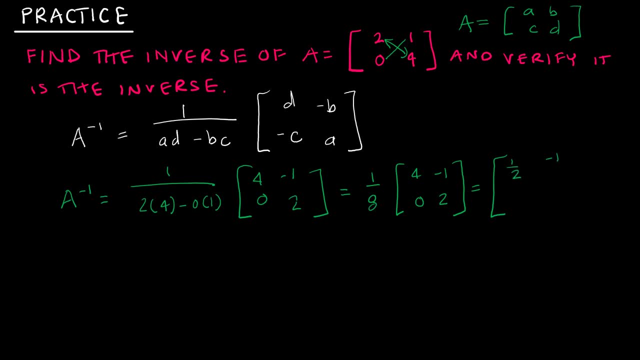 8,, which reduces to 1 half negative, 1 over 8,, 0 over 8,, which is 0, and then 2 over 8,, which is 1. fourth, So that is my inverse matrix for A. Now I'm going to verify. it is the inverse. So to: 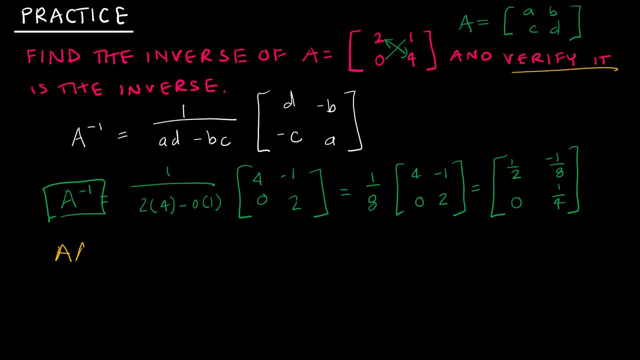 verify. I'm going to take A times A inverse and that means I have 2, 1, 0, 4, times 1 half negative: 1, 8, 0, 1. fourth, And again you can feel free to help yourself with a calculator, but it's good. 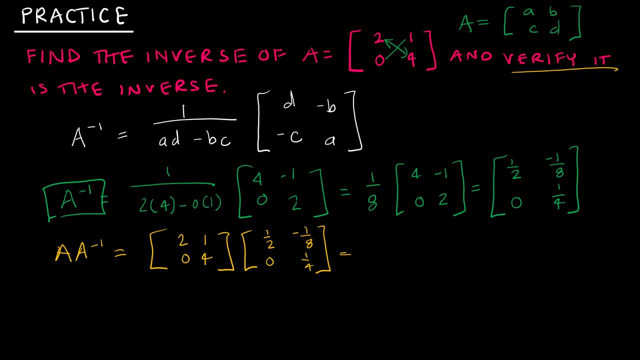 for you to do mental math. So if you can do it without a calculator, that's what you should do. So here we go. I'm going to take 2 times 1 half, which is 1, and 1 times 1 fourth. 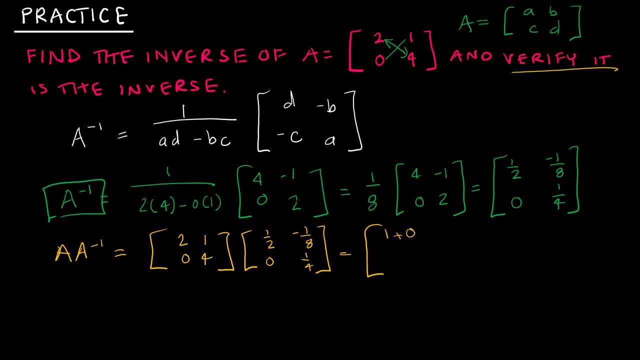 Hold on, Nope, just kidding. 1 times 0,, which is 0. I knew that was wrong. And then I'm going to take 2 times negative 1 eighth, which is negative, 1 fourth, and I'm going. 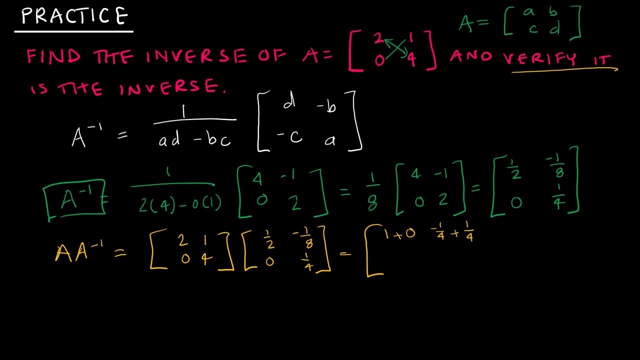 to take 1 times 1, fourth, which is 1, fourth, And that was my first row- times each column, And now I'm going to take my second row, So 0 plus 4 times 0, which is 0.. And then 0 times 1, eighth is 0,. 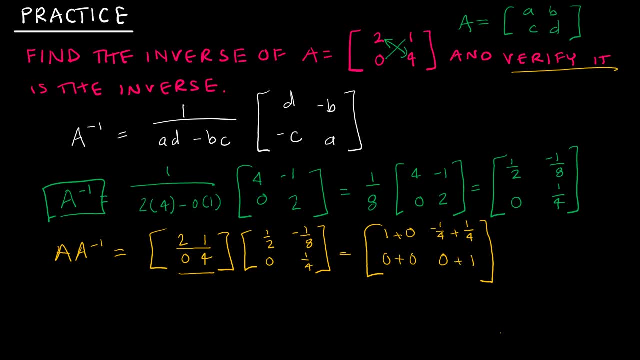 and 0,- I'm sorry- 4 times 1. fourth is 1.. So what did I end up with? 1, 0,, 0, 1,, which is the identity matrix. Now, just for fun, because math is so much fun. 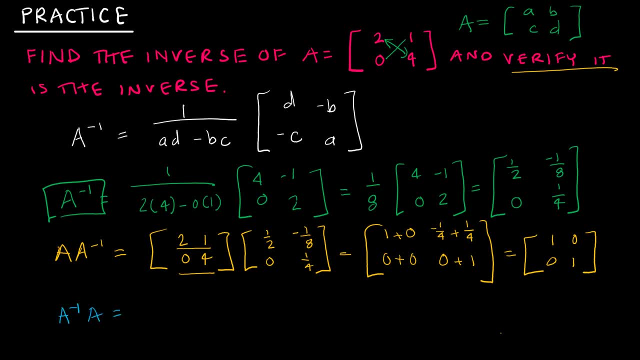 let's take A inverse times A and verify that we do in fact still get the inverse- I'm sorry, the identity. So the inverse again was 1 half negative, 1 eighth, 0, 1 fourth, And if I take that times A,